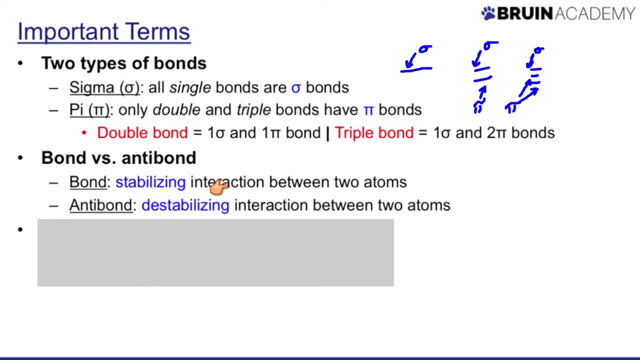 are stabilizing interactions. They lower energy, so they increase stability. It turns out that for every bond that is formed, an antibond is also formed. Now. antibonds are the opposite. They're destabilizing interactions, so they actually increase energy. And we'll write. 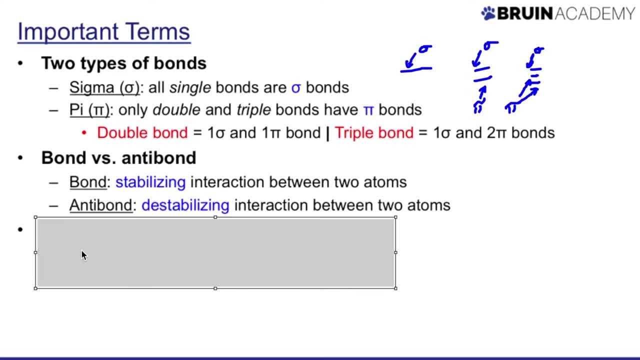 out both bonds and antibonds on our molecular orbital diagram. The last thing you should know is that a given molecule can have one of two magnetic properties. It can either be diamagnetic, which means it has no unpaired electrons, or it can be 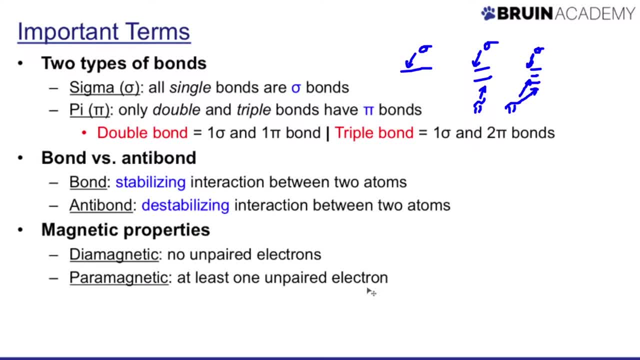 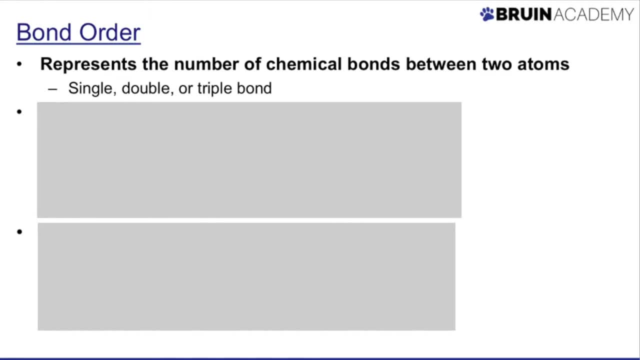 paramagnetic, which means it has at least one unpaired electron. This is something you can only determine by drawing the molecular orbital. The other thing you need to know is how to calculate bond order, And bond order represents basically the number of bonds between. 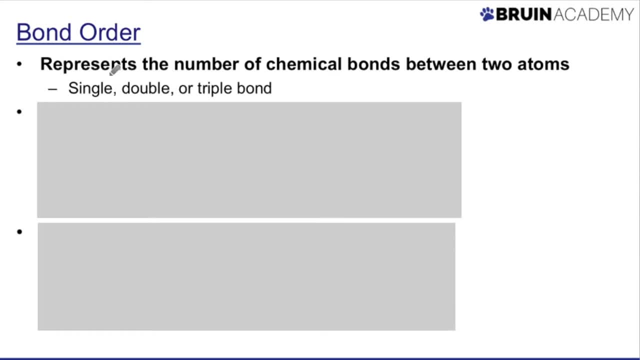 two atoms. So if bond order is equal to one, you have a single bond, If bond order is equal to two, you have a double bond, And if bond order is three, you have a triple bond. It turns out that bond order doesn't have to be a whole number. It can actually be a decimal, So it 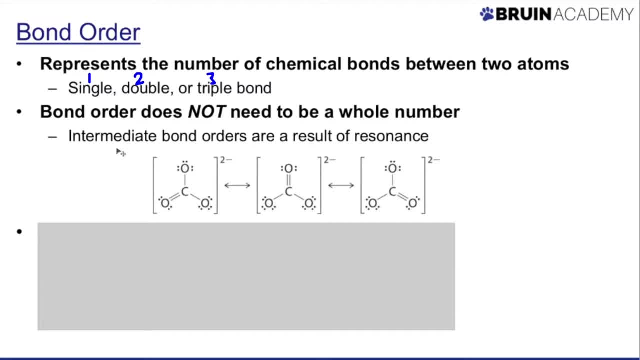 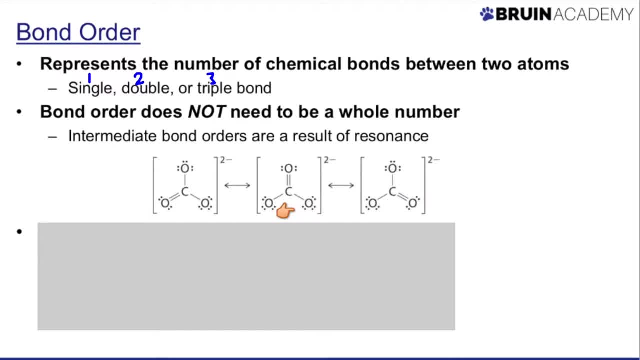 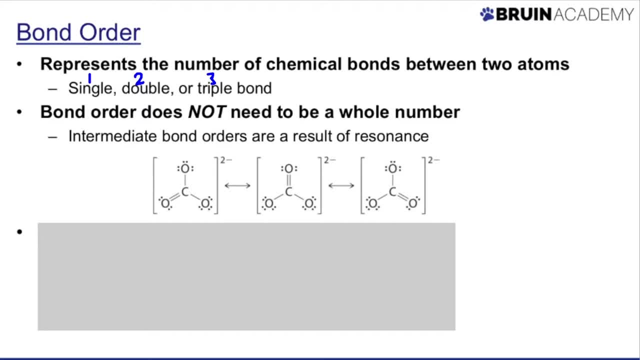 of these bonds, we would get something between one and two, And so that's how. bond order doesn't have to be a whole number, And there is an equation you use to calculate bond order, and it's the following: So bond order is simply equal to one half of the electrons found in 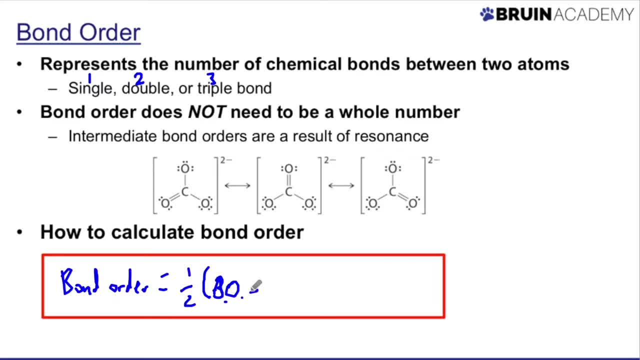 bonding orbitals, so bonding orbital electrons, minus the electrons found in anti-bonding orbitals, so anti-bonding orbital electrons. you take the sum, you count the total of bonding orbital electrons, total of anti-bonding orbital electrons, subtract them, divide it by two and that's your bond order. 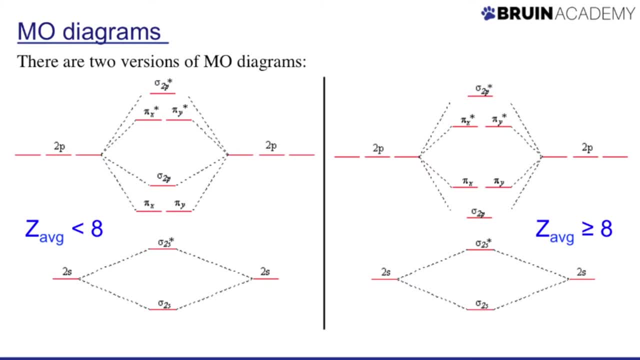 okay, so you've probably seen this before. it's in your course reader. there are two versions of MO diagrams, depending on what your atomic number is or your z. if your z is less than eight, you're going to use the left MO diagram, and so you should memorize this arrangement whenever you draw an MO. 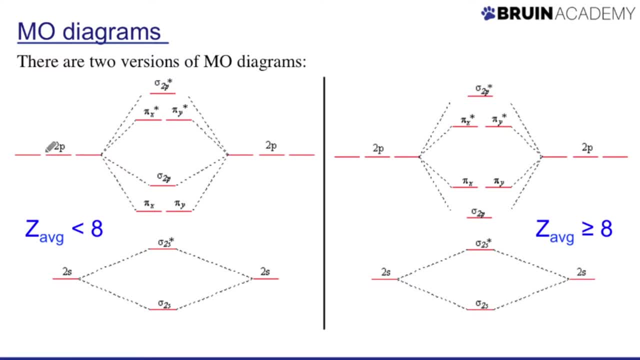 diagram. you should start with this. so start with your atomic orbitals, which is on the left and the right, with the 2s and the 2p. the 2s combine to form a sigma bond and an anti-sigma bond. remember, every time you form a bond, you also form an anti-bond, and then they also form these two pi. 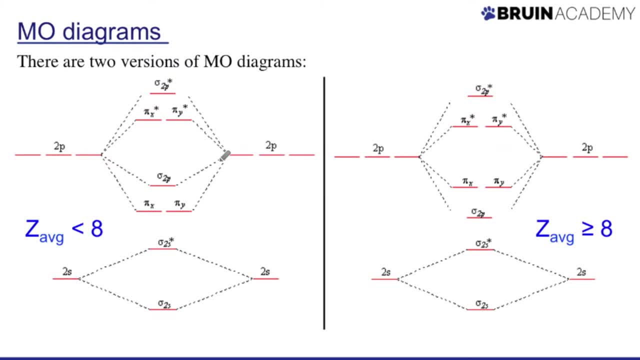 bonds as well as a sigma bond, and then you can also form an anti-bond, and then you can also form an anti-sigma. now, really, the difference between the the left and the right is this: everything else is the same. the order is switched. so, on the left, you have the sigma bond above the two pi's. 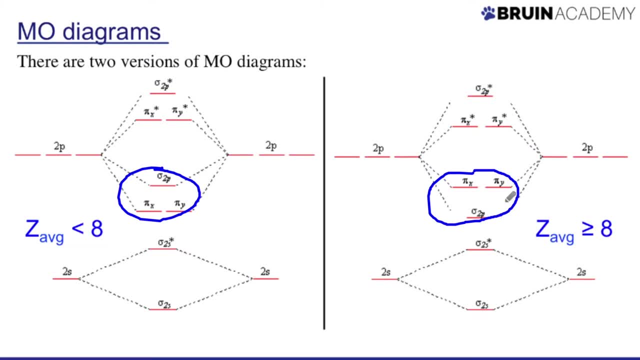 whereas on the right you have the two pi bonds above the sigma and notice that the anti-bonds are the same for both, for both sides. so really, the first step to figuring out which MO diagram to use is to calculate the atomic number, the average atomic number and sometimes the 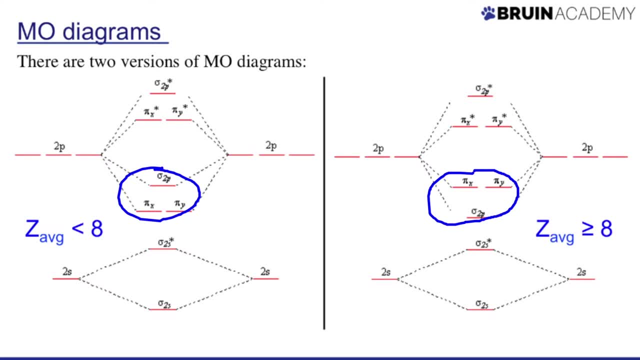 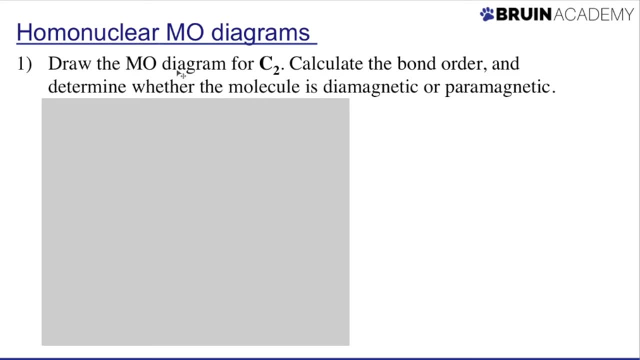 atoms are the same, in which case you only have to look at one of them. all right, so you should memorize these two arrangements, okay? so let's draw the MO diagram for C2. we're going to calculate the bond order and determine whether it's diamagnetic or paramagnetic. so the first 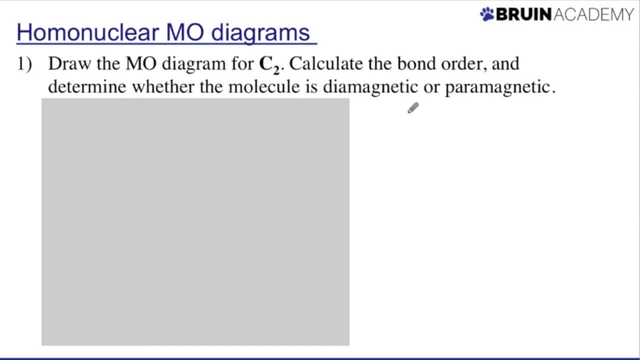 step is to figure out which version of the MO diagram to use. so we're going to figure out the atomic number of carbon, which is 6, and so, because the atomic number is 6, it's less than eight. So we're going to use that first version. So we're going to use that first version. 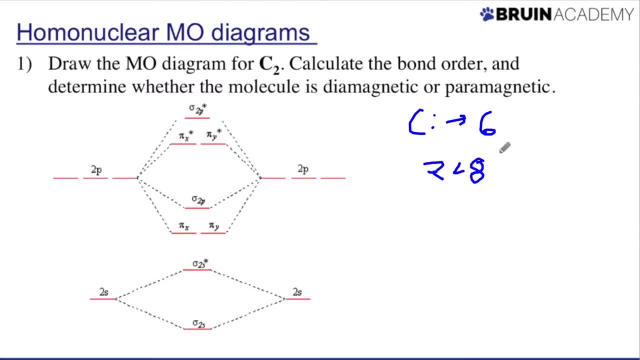 which looks as such: Carbon has six total electrons but four valence electrons, And that's what you represent in these MO diagrams. And so on the atomic orbitals which exist on the left and right, I'm going to label them as carbon, I'm going to draw on the four valence. 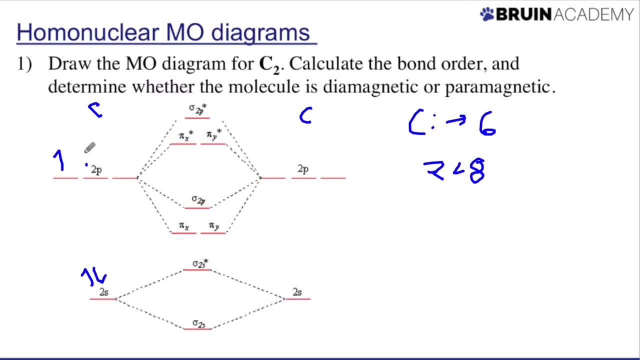 electrons, So one, two, three and four. Notice how I follow Han's rule in filling in the electrons. I do the same thing on the other side. Now that my atomic orbitals on the left and right are filled, I can fill in my MO orbitals- molecular orbitals- in the middle, And so I have a total of eight. 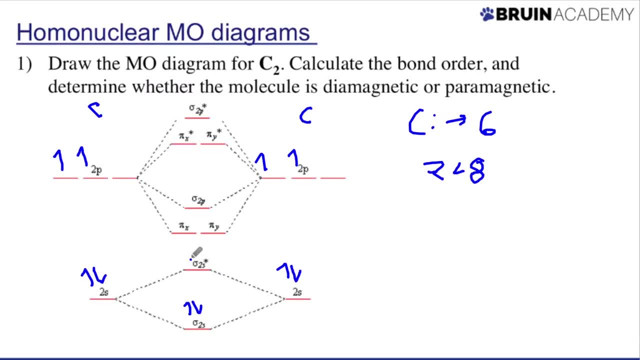 electrons. So I basically fill them as such: One, two, three, four, five, six. Notice how I fill these guys in Seven, eight. This is my MO diagram for carbon. To calculate the bond order, I simply take one. 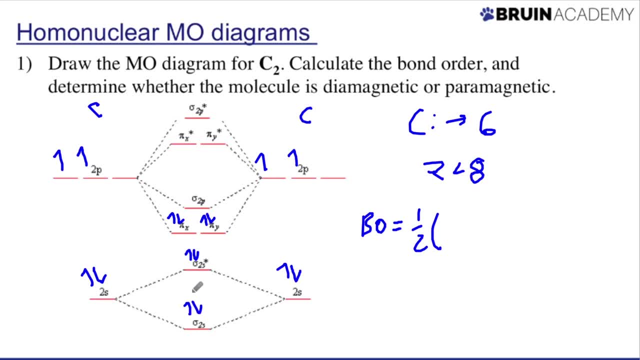 half of the electrons in bonding orbitals, which in this case is two, four, six, And I subtract by the electrons in the antibonding orbitals, which are the ones that are asterisked, So that's two, And that gets me a half of four, which is two. So really, what that tells me is that the carbons 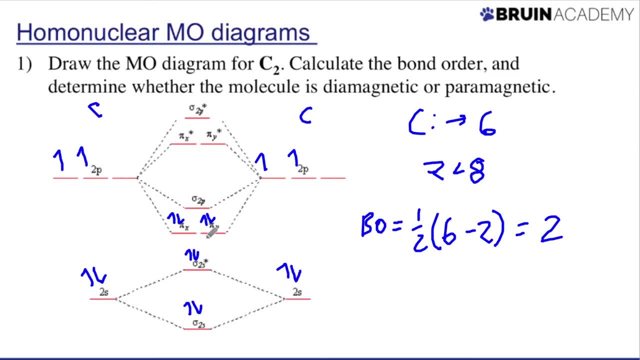 are connected by a double bond, And here you can look to determine whether it's diamagnetic or paramagnetic. You just look to see if you have any unpaired electrons. Here every electron is paired, So we call it diamagnetic And that's it. So that's for C2.. So let's try it for a different. 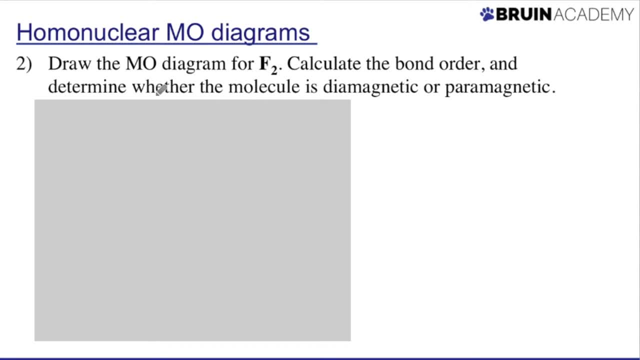 example F2.. So we need to calculate the bond order and determine whether the molecule is diamagnetic or paramagnetic. And so here, the atomic number of fluorine is nine, And so it's greater than or equal to eight. And so we're going to use the second version of the MO diagram, which is the 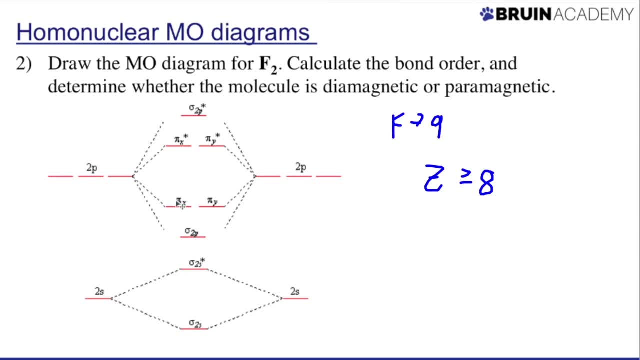 following is lower than the pi, 2p, x and 2py, And we just fill in the electrons as usual, And so for fluorine the number of valence electrons is 7. So I fill that into the atomic orbitals. 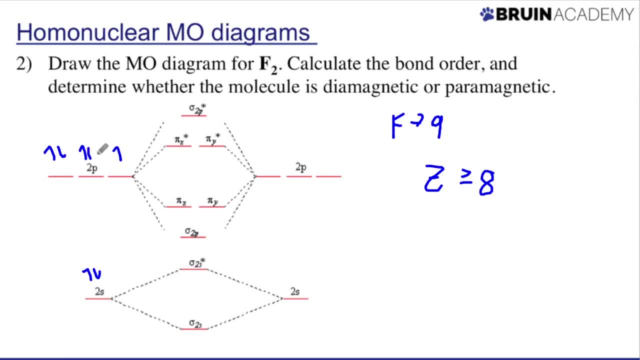 on the left and right, So 1,, 2,, 3,, 4,, 5,, 6, 7.. This is fluorine. I also have a fluorine on the right: 1,, 2,, 3,, 4,, 5,, 6,, 7.. 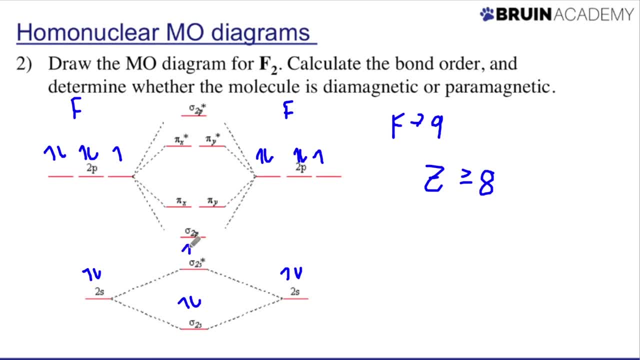 In total I have 14 electrons, so I fill them in as such: 1,, 2,, 3,, 4,, 5,, 6,, 7,, 8,, 9,, 10,, 11,, 12,, 13,, 14.. 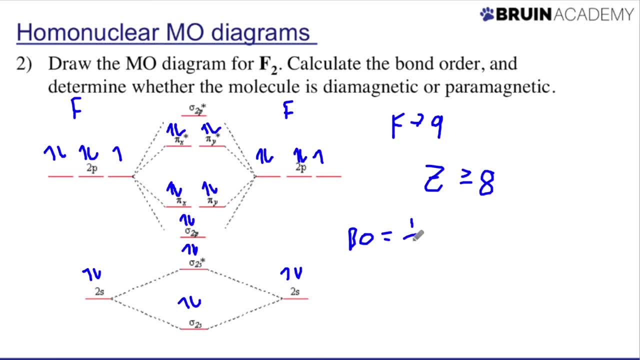 And so if I'm going to calculate the bond order, I simply take the number of electrons in bonding orbitals- non-asterisk orbitals, So that's 2,, 4, 6, 8, subtract by the electrons in antibonding orbitals. 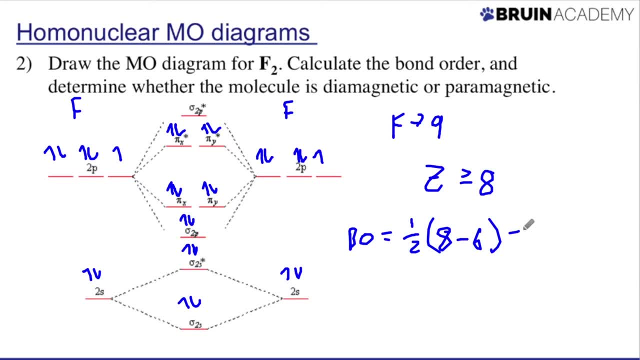 which is 2,, 4, 6.. A half of 2 is 1.. And so Fs are connected by a single bond, And here all the electrons are paired, so it would be diamagnetic. All right, and finally, 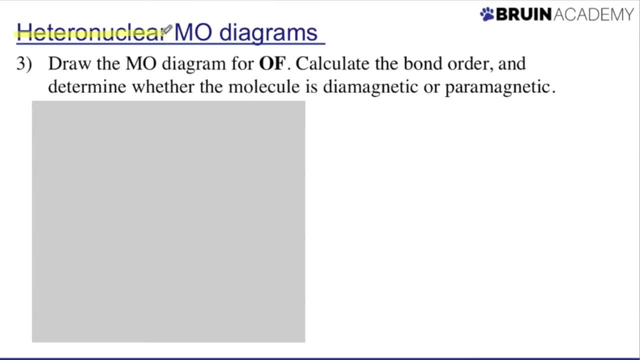 an example of a heteronuclear MO diagram, meaning two different elements bonded together. Draw the MO diagram of OF, calculate the bond order and determine whether the molecule is diamagnetic or paramagnetic. So here's the slightly tricky thing about heteronuclear. 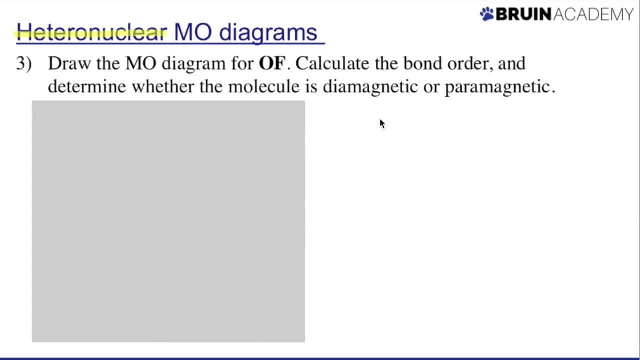 So the first thing you would do is the same as you would, the same first step you'd always do, which is to calculate the Z. And here the elements are different, so you need to calculate the average Z. So for oxygen, the atomic number is 8.. 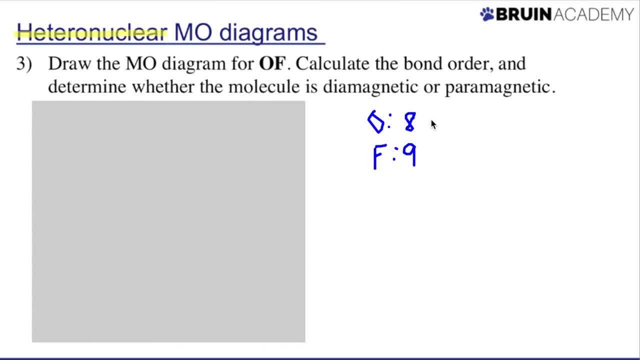 For fluorine, the atomic number is 9.. The Z average is the mean of these two numbers, which is 8.5.. That is greater than or equal to 8, so we use the second version, And so you might be tempted to use a version. 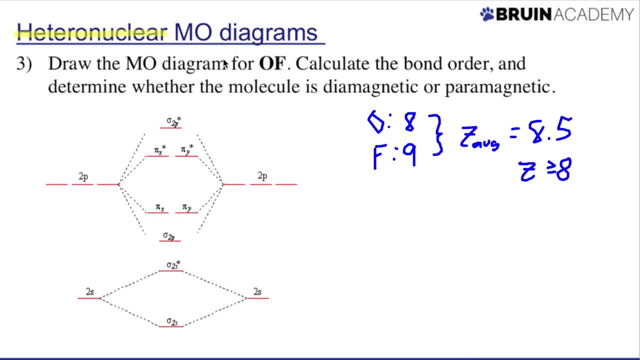 that looks like this: It turns out that for heteronuclear MO diagrams there is a bit of asymmetry, because the two atoms are different and so the energy levels of the atomic orbitals are not going to be the same. So instead, what it's going to look like: 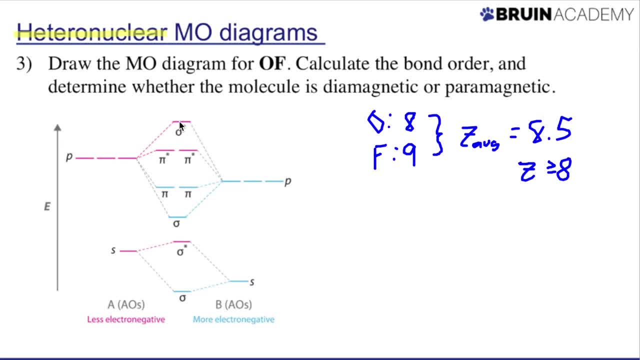 is something like this, where the arrangement of the MO diagram, the molecular orbitals in the middle, is the same, but one of the one of the atomic orbitals is lower energy than the other, And the one that is lower energy is the one that's more electronegative. 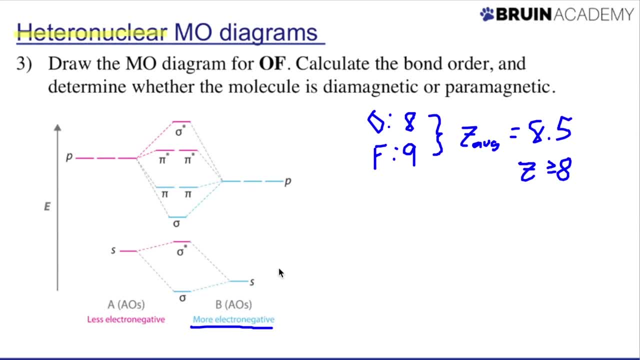 So you always put the more electronegative element on the side where the atomic orbitals are of lower energy, And here between O and F. F is more electronegative, so it goes on the right. O is less electronegative and it goes on the left. 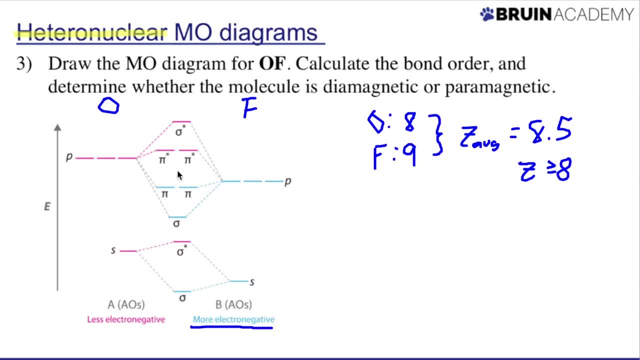 Once you do this step, everything's exactly the same as what we've done for the homonuclear. So oxygen has a total of six valence electrons, so I put them in one: One, two, three, four, five, six.